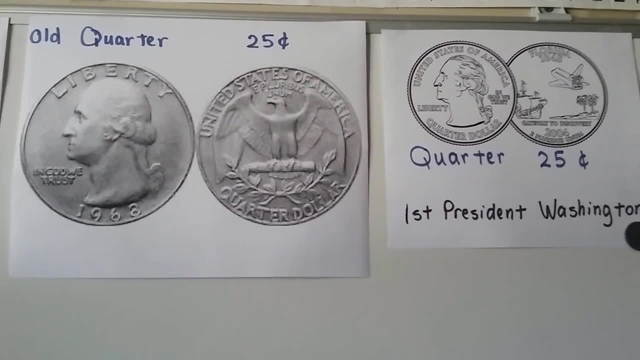 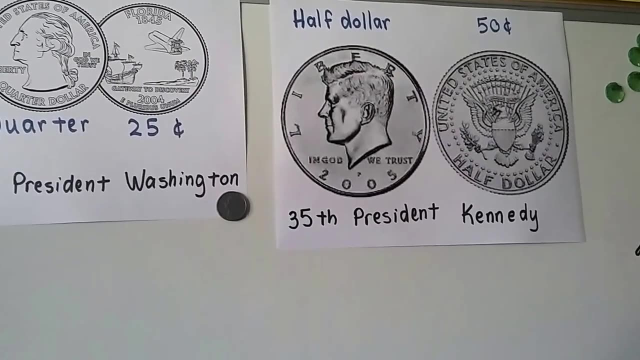 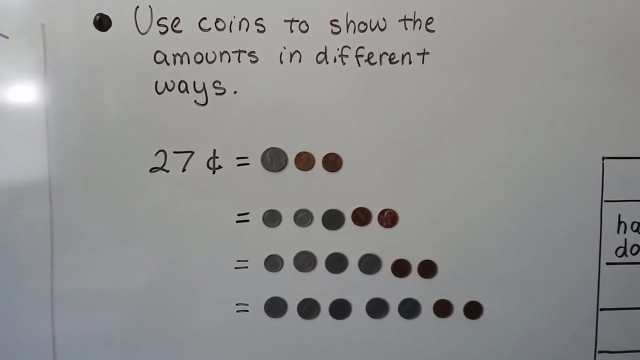 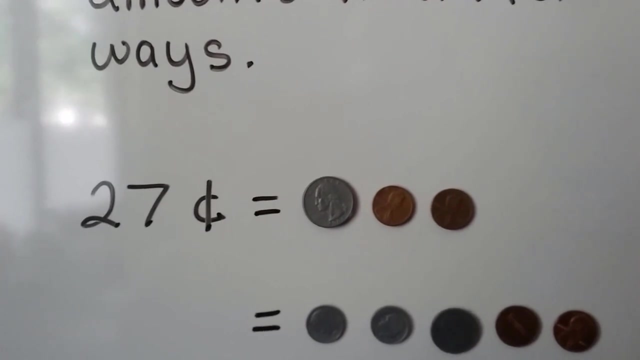 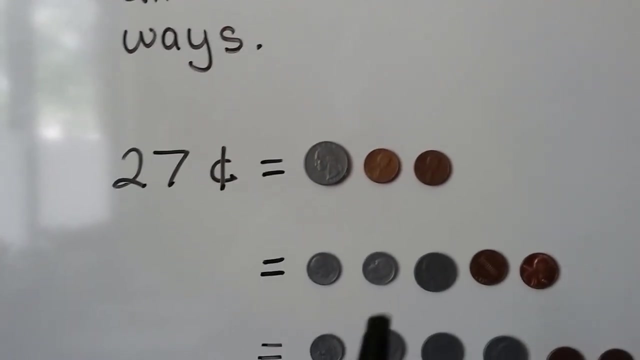 quarters. either way, they're worth 50 cents. that would be one quarter with 25 cents. then we have the half dollar. it's 50 cents. okay, we can use coins to show the amounts in different ways. 27 cents- well, that would be equal to a quarter and two pennies. that's a twenty-five. 26, 27 cents, and because two 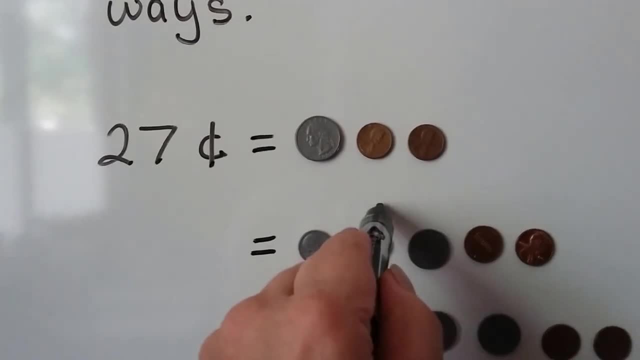 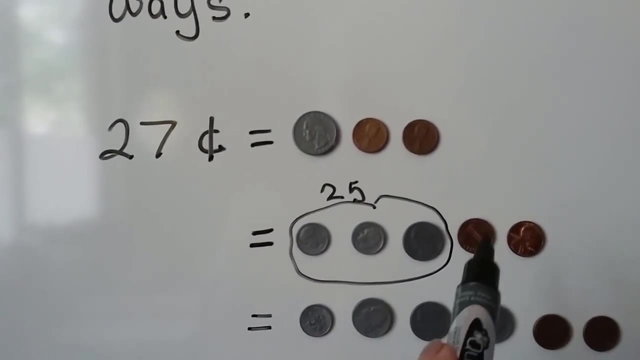 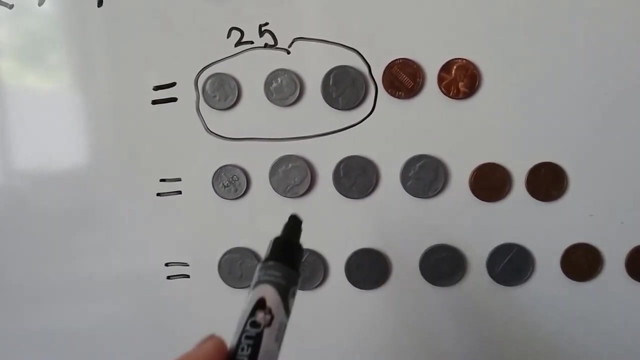 dimes and a nickel is also the same thing as a quarter. this right here is the same thing as 25, it's two tens and a five. we have 25, 26, 27 and we can also do a dime and one, two, three nickels and two pennies. do you notice? because it's 27 we. 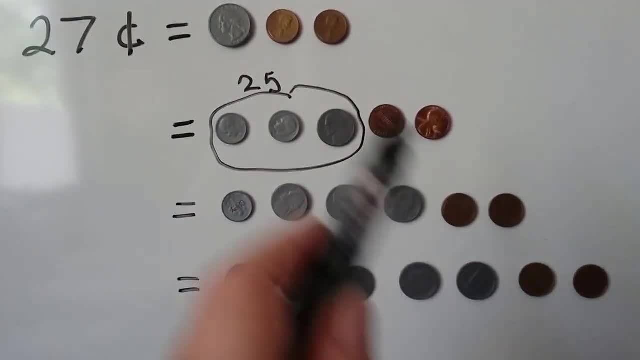 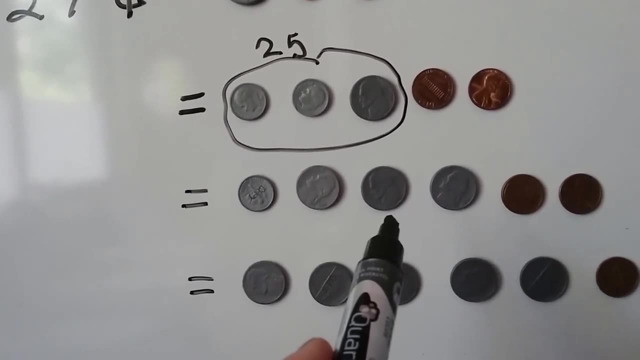 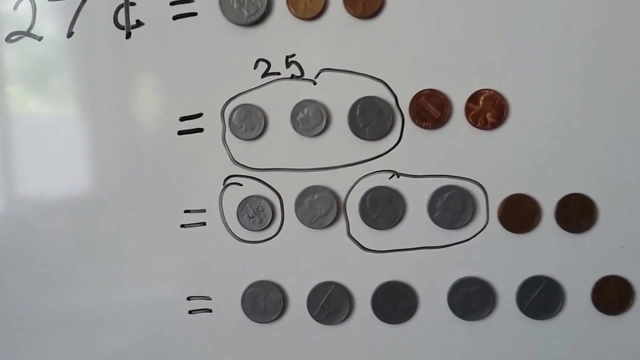 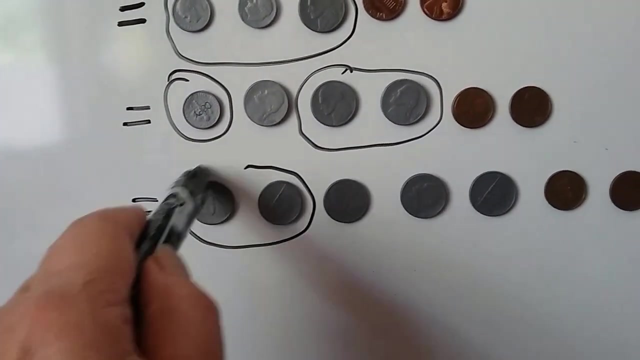 always have the two pennies there to make the six, seven. we have ten and five and five and five. this makes a ten, that's a ten. and then we have the five, 25, 26, 27. we could also do all these nickels. two nickels make a dime, that's. 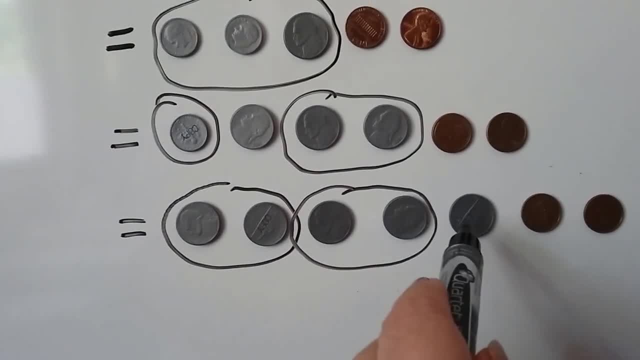 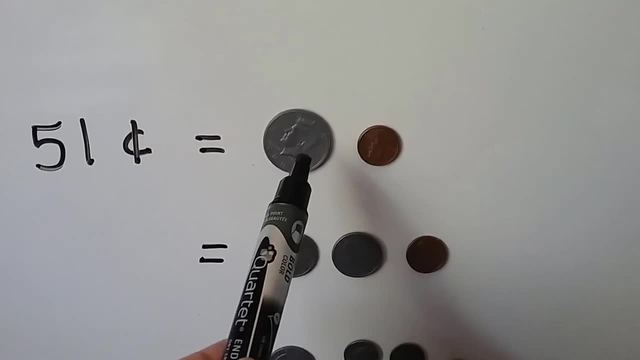 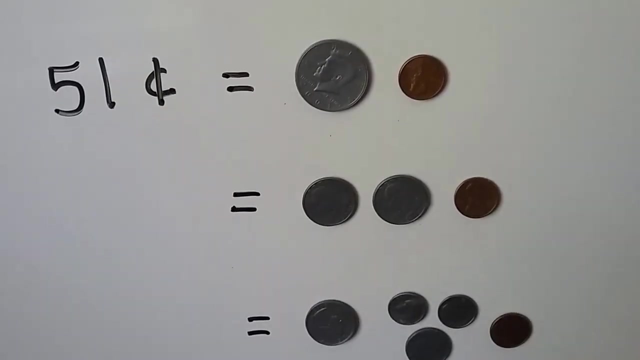 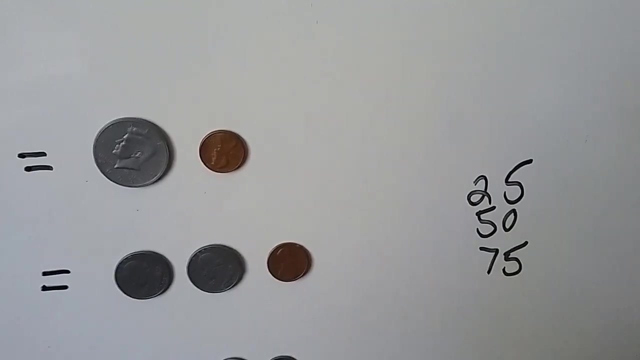 10, 20, 25, 26, 27 for 51 cents. we could use a half dollar, which is 50 cents, and a penny. we could also use two quarters, because when we count by 25 we say 25, 50, 75, right when we 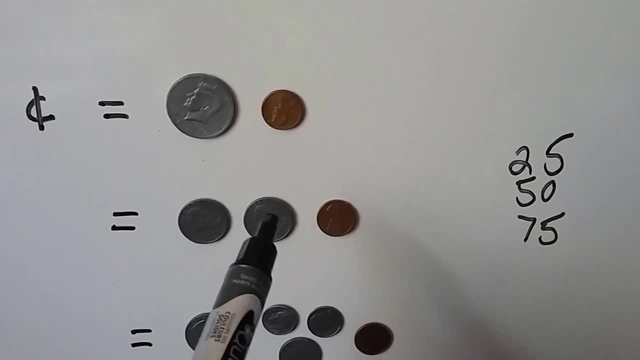 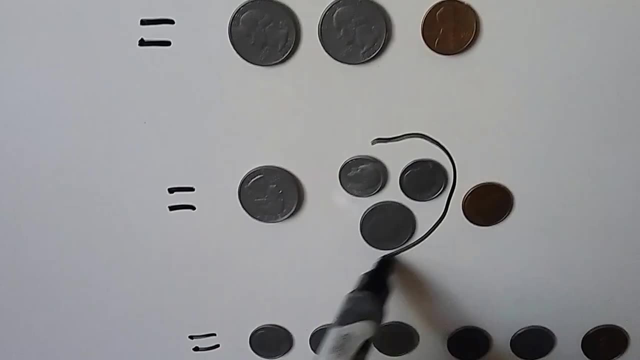 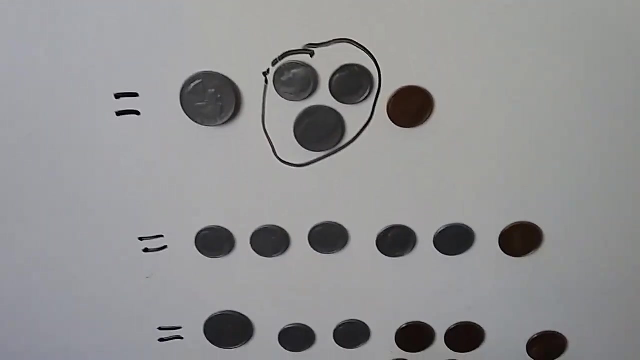 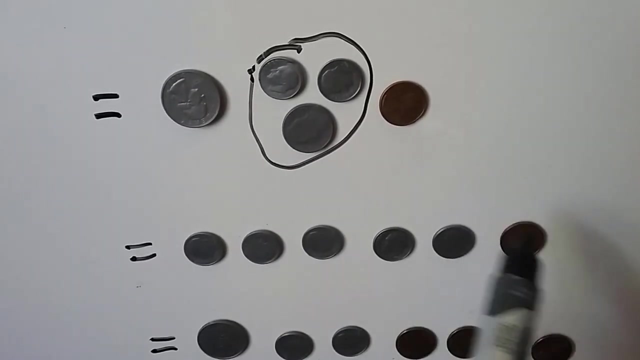 count by 25 when we count quarters. so we have 25, 50, 51. here we have two dimes and a nickel, and remember that's 25. so we can count by 25 s again 25, 50 one. here we have five times. we can count by ten's: 10, 20, 30, 40, 50 one. here we have a quarter. 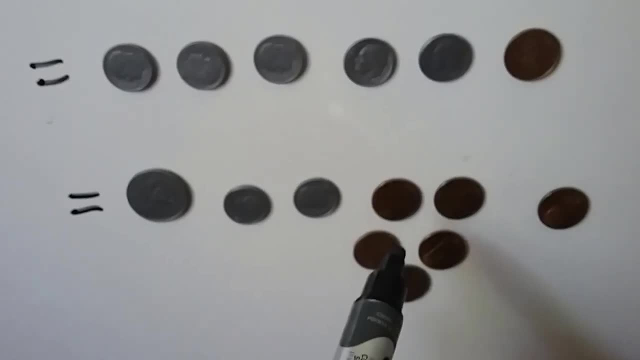 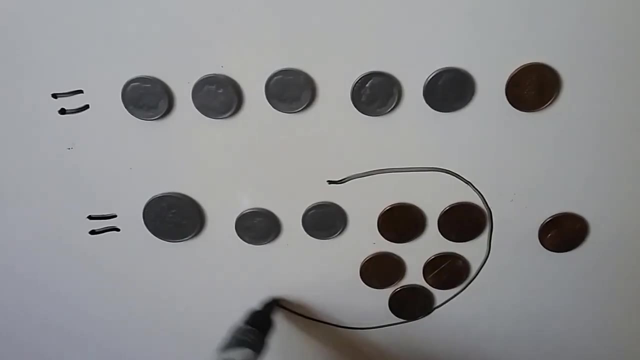 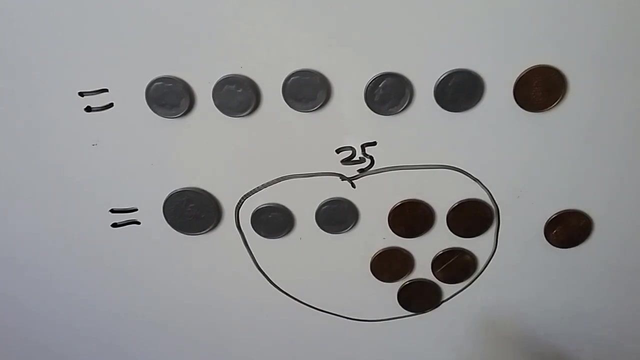 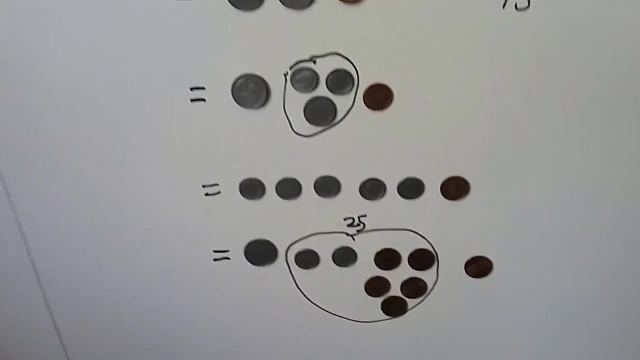 that's 25 cents. we have two dimes and look, we have one, two, three, four, five, six pennies. well, this- two dimes and five pennies- makes a 25, doesn't it? it's the same thing as a quarter, because the five pennies is the same thing as a nickel, it's five. so now we have 25, 51, see we. 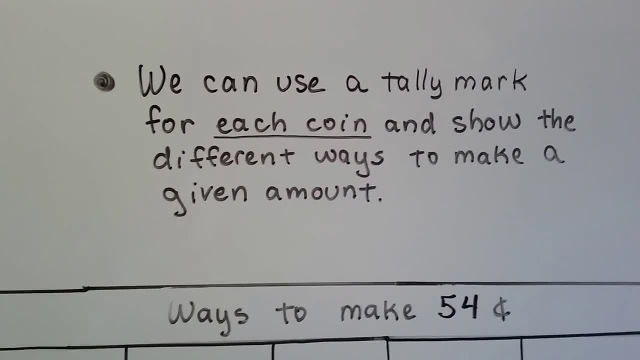 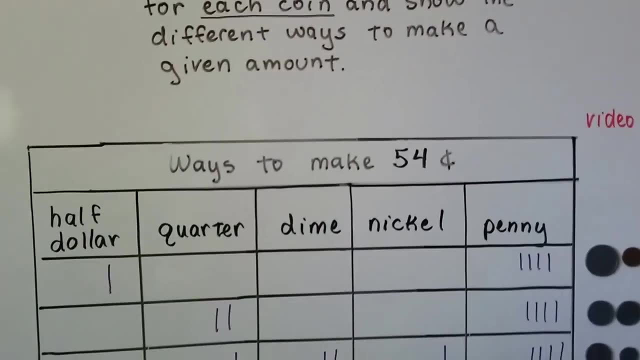 can use a tally mark for each coin and show the different ways to make given amount. now, if you remember from video 4.2, we made a table but we actually wrote the number in the box and we put zeros if we didn't use any in this table. 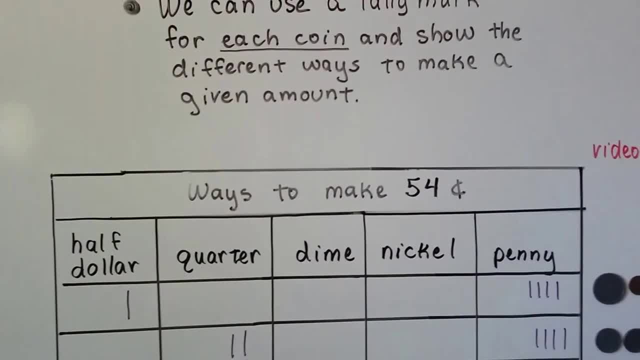 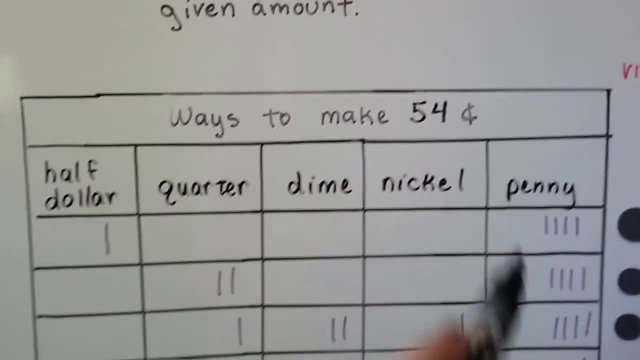 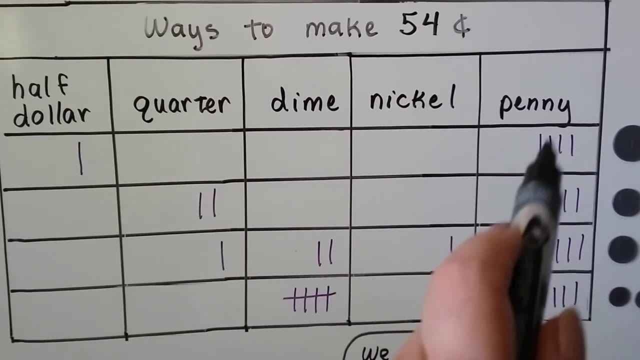 we're gonna use a tally mark that's a line for each coin, and we're gonna show the different ways to make a given amount. so we need to make 54 cents. so what we can do is we can use a half dollar- that's 50 cents, and 4 pennies. 1, 2. 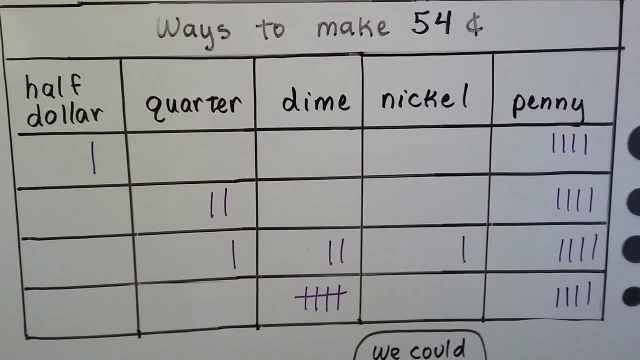 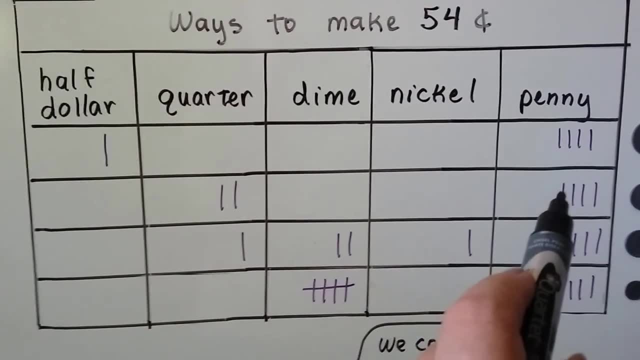 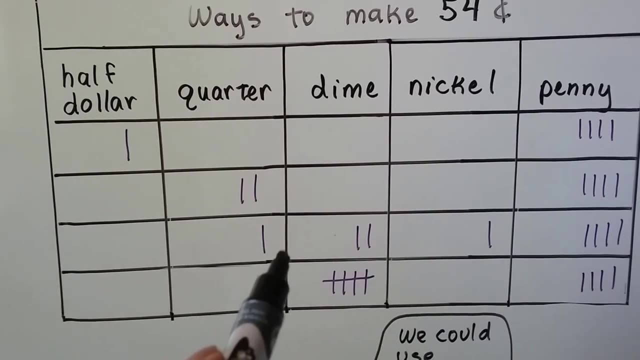 3, 4. we use a tally mark for each coin. that would be 54 cents. we can also use two quarters, 25, 50 and 4 pennies. see, that would be 54, because 2 dimes and 1 nickel is the same thing as a quarter. we could use a quarter, 2 dimes and a nickel. 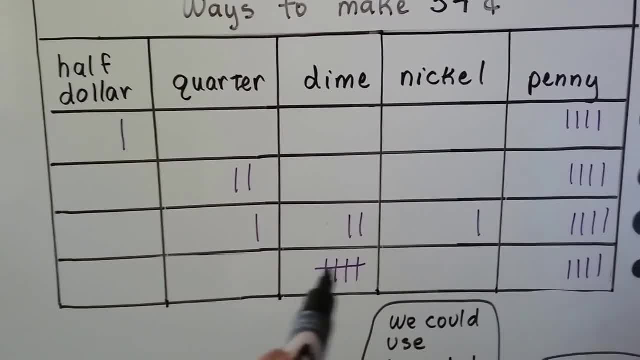 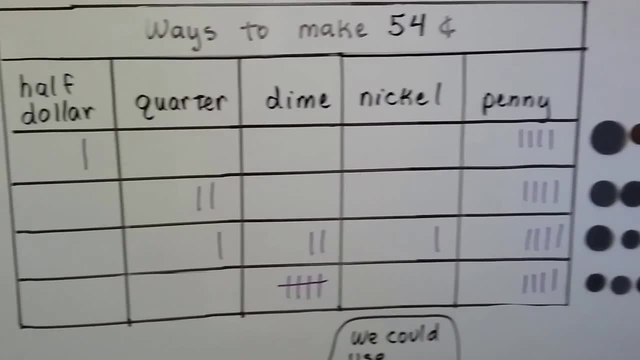 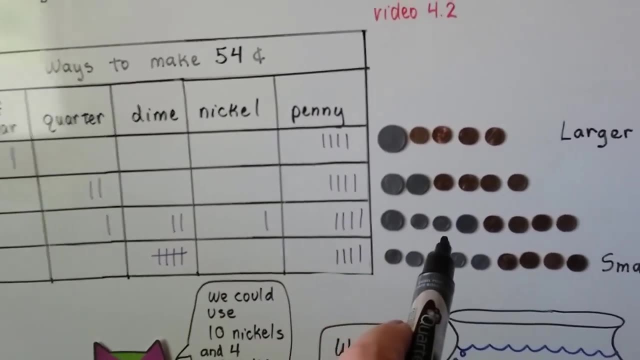 and 4 pennies. we could also use 5 dimes, 5 tens. that would make 50 and then 4 pennies would make 54. so if you look at the tally table and the coins that we used, what do you notice? this is valued at 50. 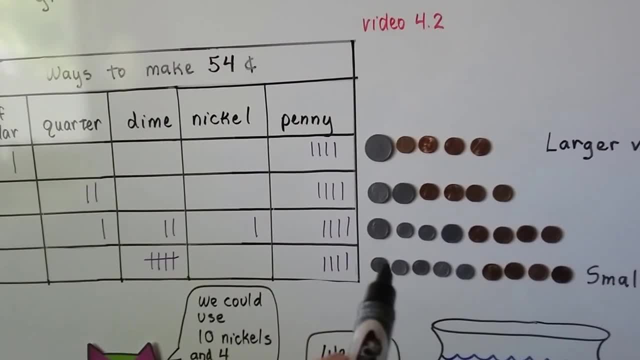 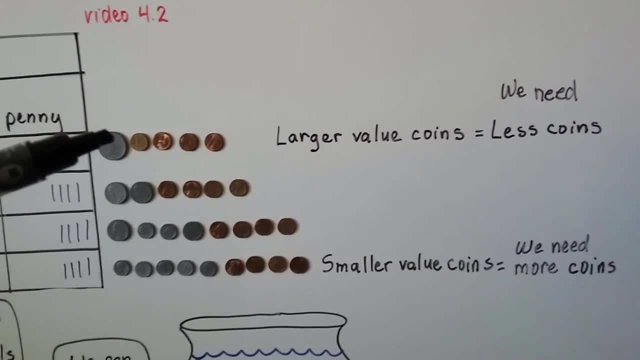 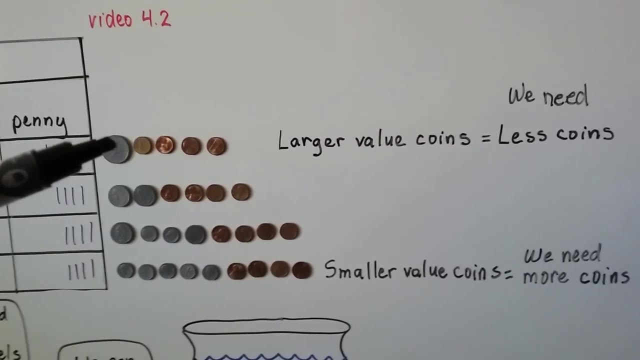 and each of these coins start getting smaller and smaller, don't they? until these are just valued at 10 and 1 down here? well, the larger value coins means we need less coins. if we've got big coins that are worth more, we don't need as many the smaller value coins, like these dimes or nickels. 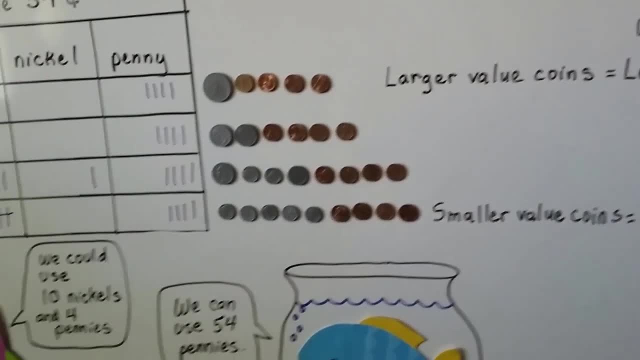 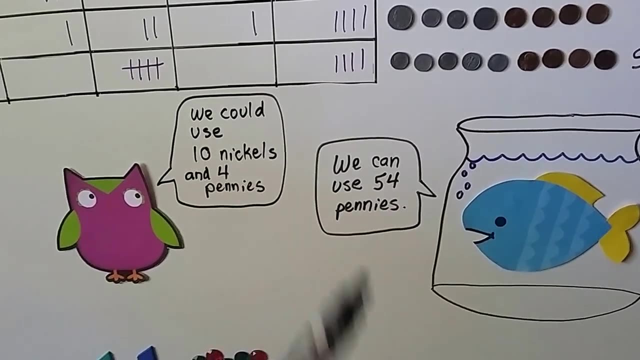 we're gonna use the smaller value coins, like these dimes or nickels. we're gonna need more coins. see, we can use 10 nickels- that would be 50 cents- and 4 pennies. we could also use 54 pennies, couldn't we? that would be a big handful of change.